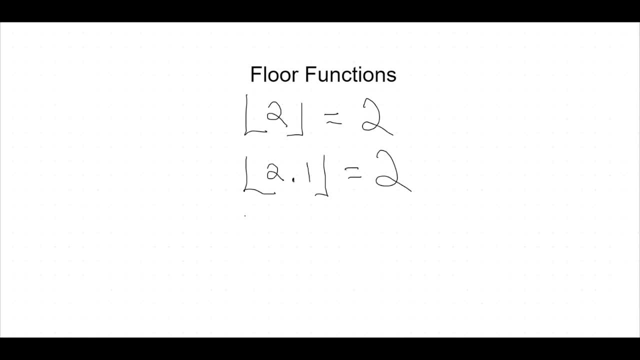 Alright, let's try something else. What if we put 2.9 into the number 2? 2.9.. Can you guess what it will be? Well, if you guessed that it was 2, you'd be correct. That's right, It's all 2.. 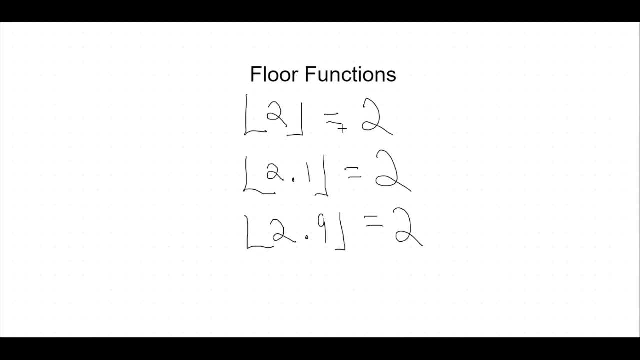 So does it just always spit out 2? No, It will spit out other numbers too. So let's try: how about 3.001.. What will it spit out then? Well, it turns out then the output will be equal to 3.001. 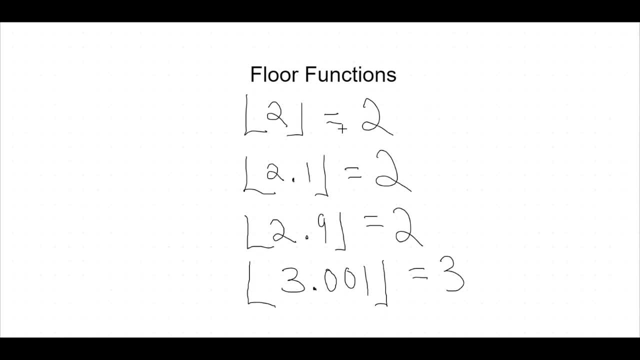 Hmm, Okay, I think it's about time we actually get the actual definition. So here we have the official definition for floor functions. The floor function of a real number, x, is defined to be the greatest integer less than or equal to x. So x is basically the input that we're plugging in. 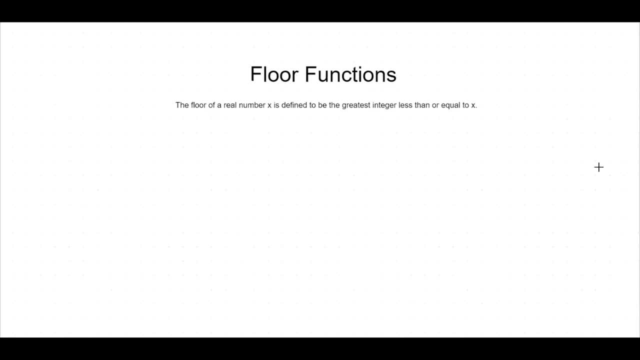 And what it's spitting out, or the floor function is spitting out, the output will be the greatest integer, less than or equal to x. So when we had 2.1, when we had the floor of 2.1,, that is. 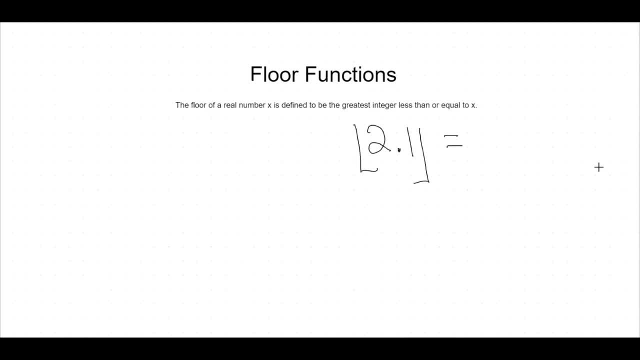 the greatest integer that was less than 2.1 was 2.. Right, Because the next greatest integer than 2 would be 3, and that's greater than 2.1. So you can't have it greater. it must be less than or equal to. 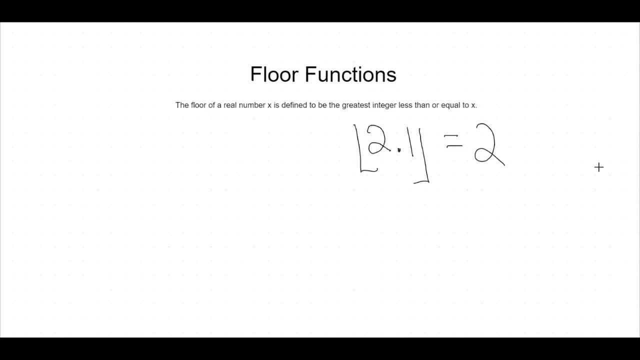 So then the greatest integer would be 2.. And since the condition is less than or equal to, when we evaluated the floor of 2, it was still 2,, right, But once we got to 3.001, well, now the greatest integer less than this is no longer 2,, because 3 is also less than this number, right. 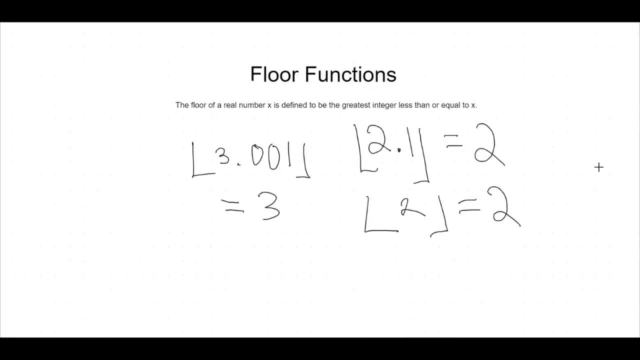 So then this comes out to becoming 3.. So that's basically the definition of floor functions.